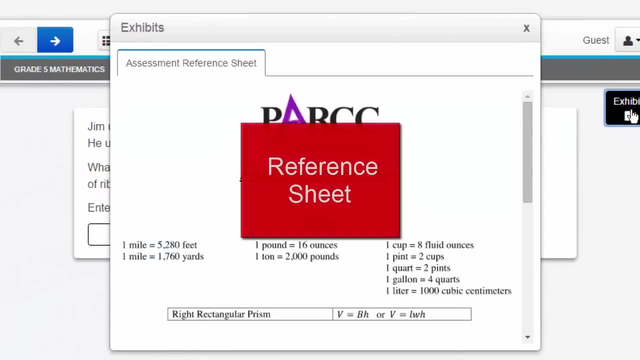 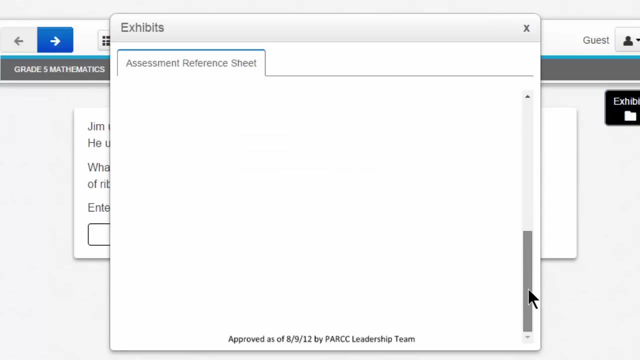 Click on that. Clicking Exhibits will pull up a reference sheet. This is information you may need to complete the test. The reference sheet here shows some unit conversions as well as a formula. Scrolling through helps you access all of the different reference materials that you may use. This sheet is for your use If. 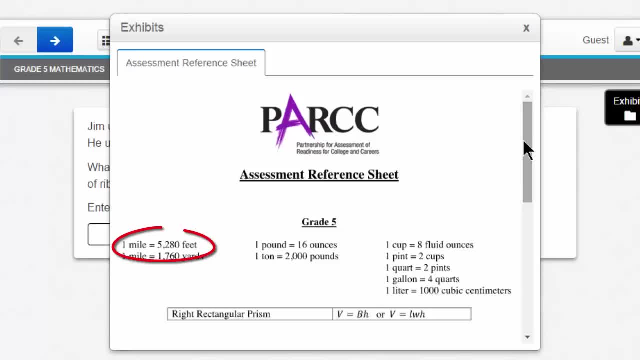 you do not remember the conversion between a mile and feet? don't worry, The reference sheet will show you. Use it as you need to, When you're finished with it or if you're not using it. click X. You can access exhibits. 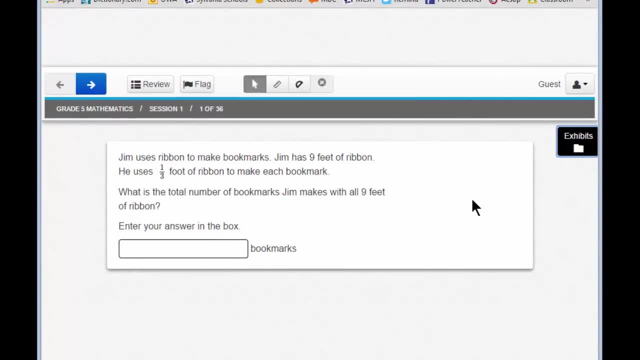 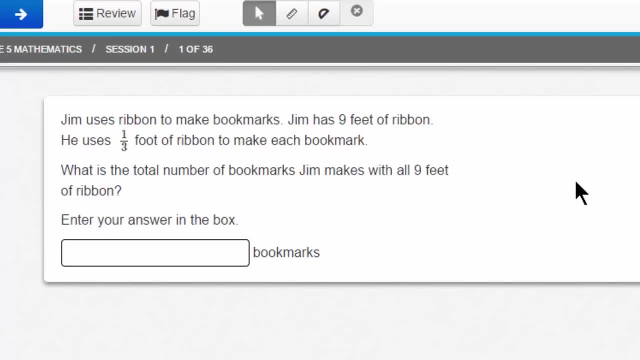 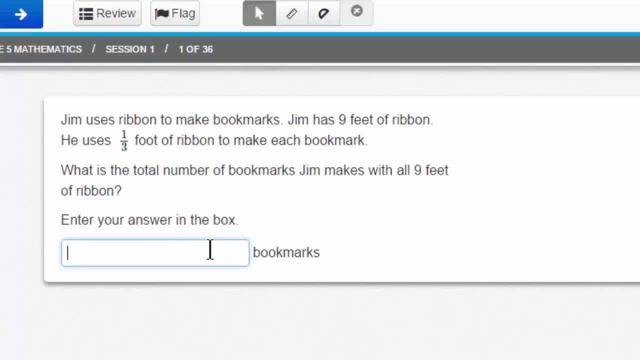 in the box and you'll see that it highlights Type 27 and your answer is entered. Remember you don't need to click submit or save to enter your answer. It's entered and you're ready to move on. Be very careful with answering this question, Since it is not multiple choice. 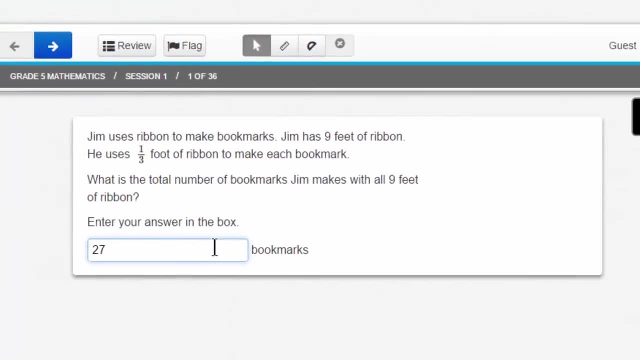 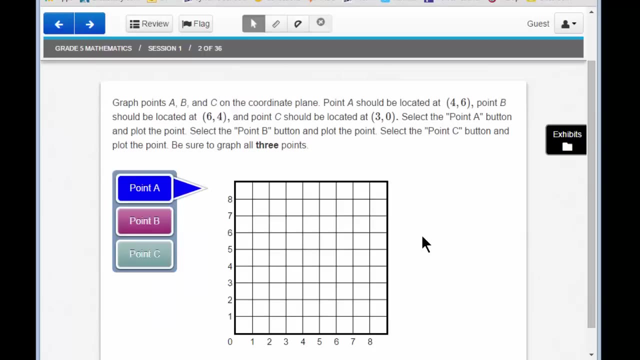 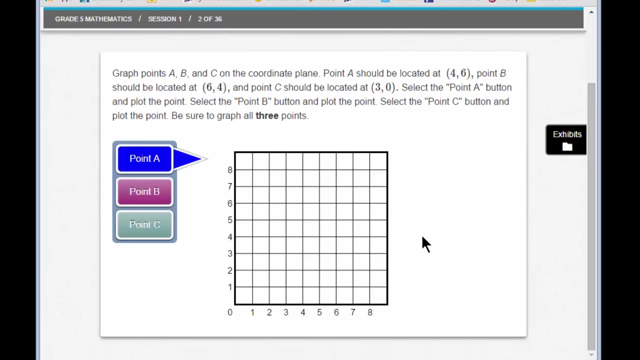 you must type correctly. Let's move to item number two. Item number two looks quite different. Let's scroll to make sure we can see all of it. This is a graphing item and as you read, you'll see that it asks you to graph three points. 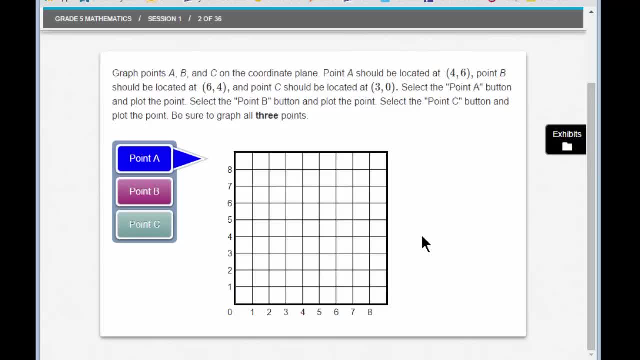 A, B and C on the coordinate plane. It gives you the coordinates to plot the points. Read the last sentence. Be sure to graph all three points. The three is bold and that tells you that you must answer three questions. Let's try. 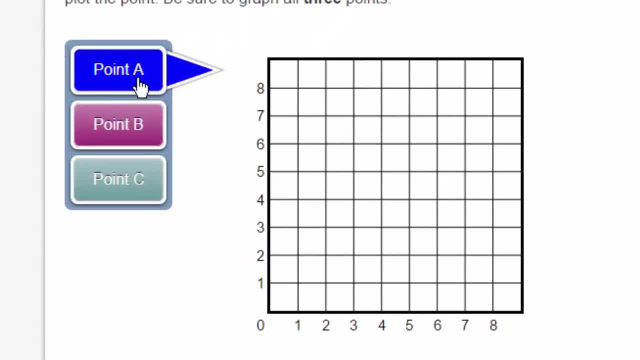 to plot point A. Point A has an arrow next to it and that means that we're ready to plot it. If we were plotting point B, the arrow would be there. Clicking on point A shows that we're plotting point A and it will be blue. That point is at 4, 6.. Let's say I've 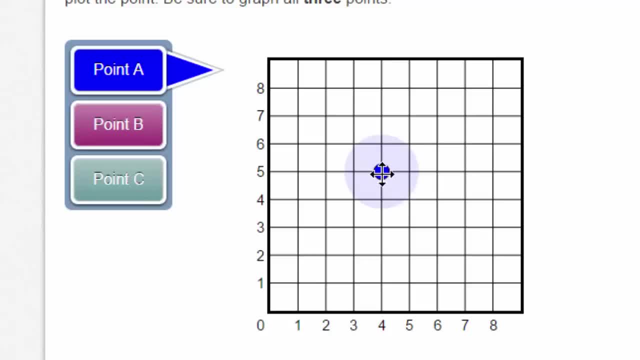 clicked there, but that's not where I wanted to plot the point. Click on the point again and it goes away. Then I can re-plot. If I'm ready for B, I'll click B. When I'm ready for C, I'll click. 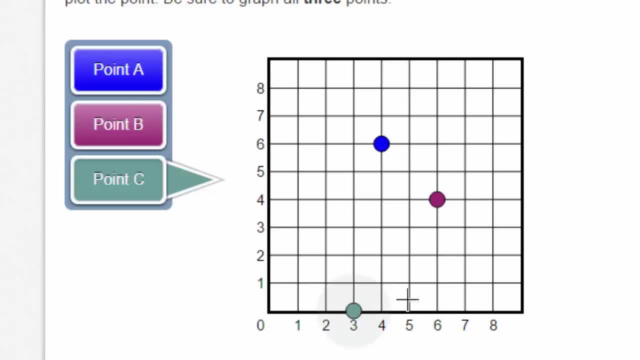 C. Once I have answered all three questions and plotted all three points, I'm finished. Be sure that you answer the entirety of the question and don't move on until you have. If you've decided that you made a mistake with point A and you wish to re-plot, do not forget to. 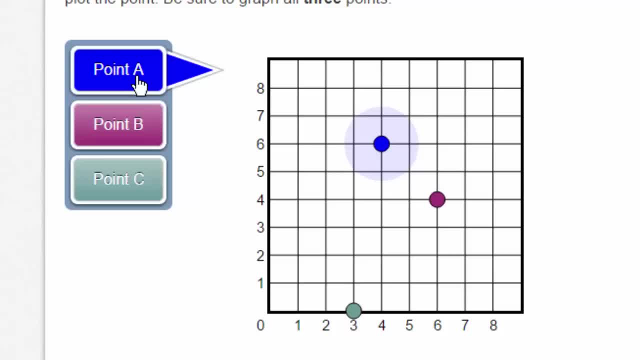 click on point A, Otherwise you won't be able to move it. Clicking on these buttons to the left gives you the power only to address that particular point: C, B and A. Why don't you try it for a moment? 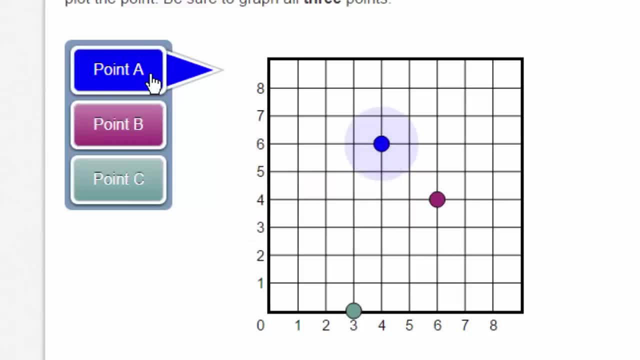 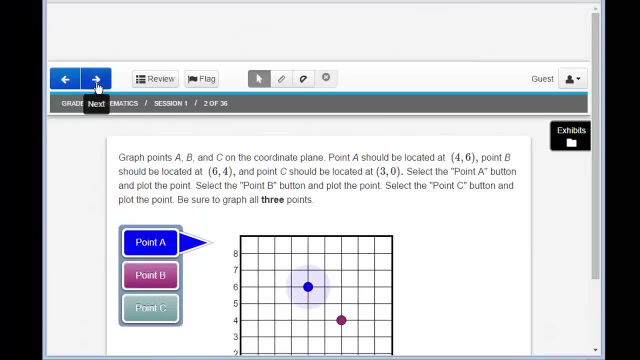 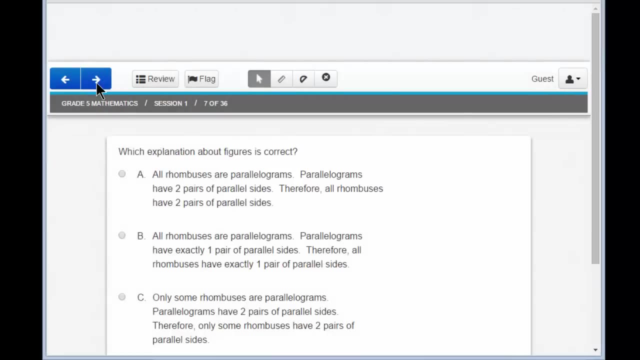 Are you ready to move on? Excellent, Then let's use the navigation buttons to move forward to item 7.. Do you remember how to notice if you're on item 7? You'll see that right here. 7 of 36.. 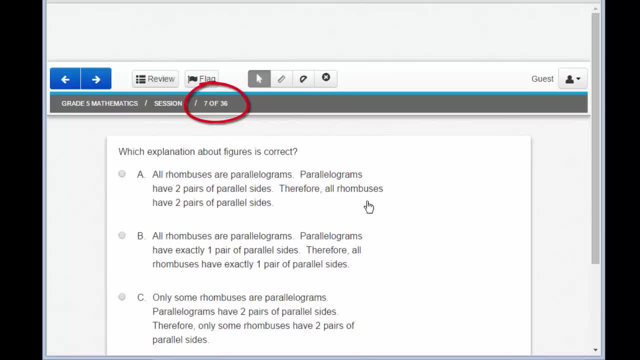 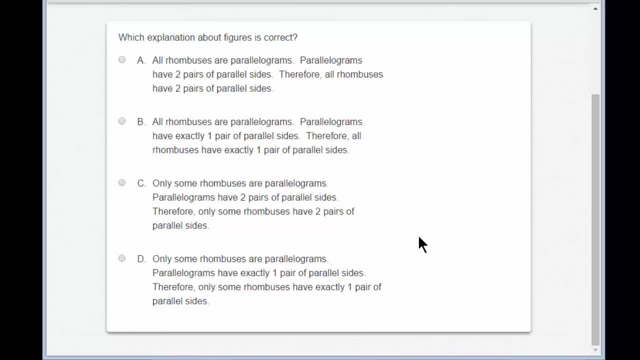 Item 7 is a simple multiple choice question. Which explanation is best for you? Maybe one of this? This- Yes about figures- is correct. This looks the same as any ELA item. You'll see a little circle and when the pointer hovers over, you can click in the circle to answer. 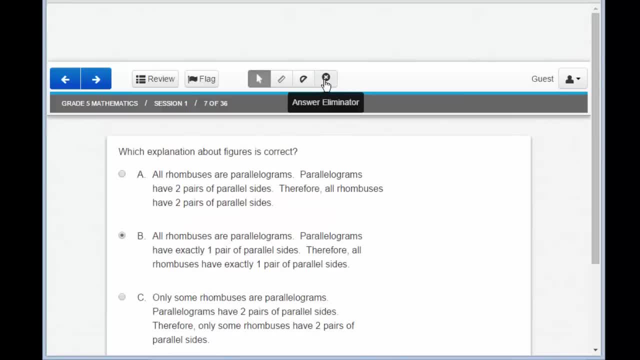 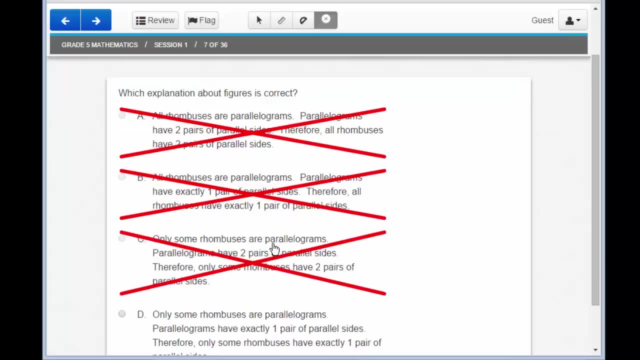 your question. You can also use the answer eliminator here in the toolbar to cross out items that you know are incorrect. Remember that clicking on the X makes it go away and you can answer whatever you'd like. Use the answer eliminator to cross out items you know are incorrect When you're ready to. 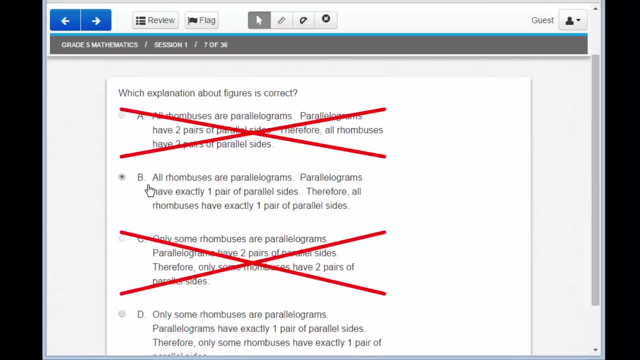 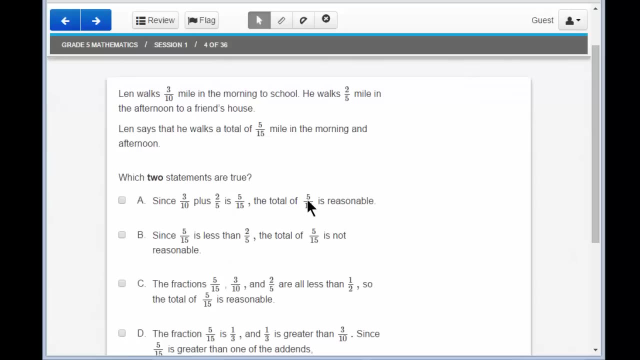 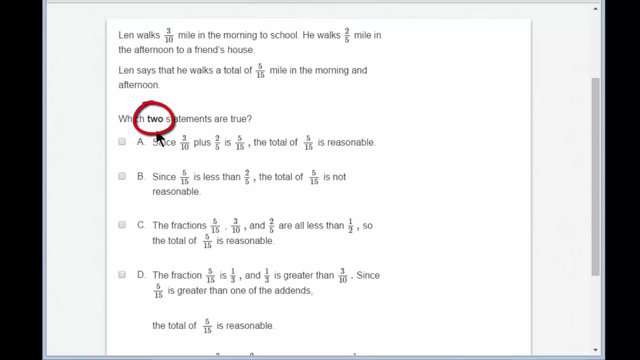 answer. select the pointer again and select in the circle. Let's move back to item number four to see something else we've seen already. Do you see anything else? Do you notice what's different? Item 4 is asking which two statements are true, See. 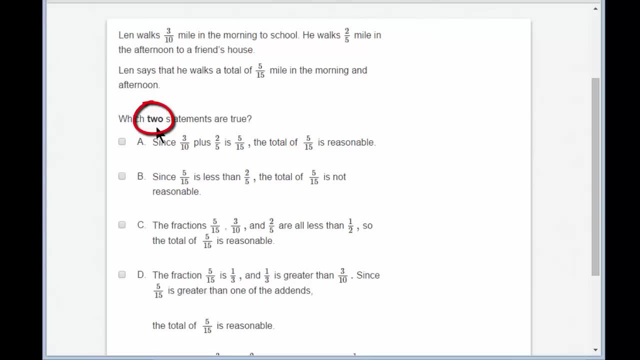 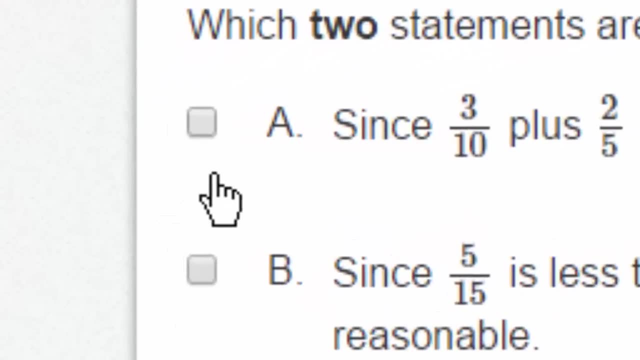 the bold. Remember that I've told you. the bold will indicate how many answers you must give And you should remember from the ELA tutorial that these boxes appear instead of circles. The boxes show you that you must answer two of these items, not simply one, And as you scroll down you can see that five options exist. 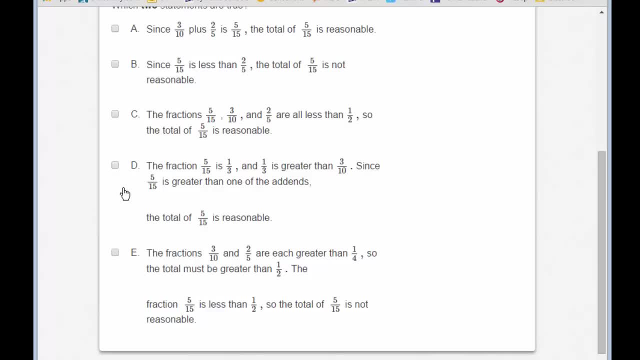 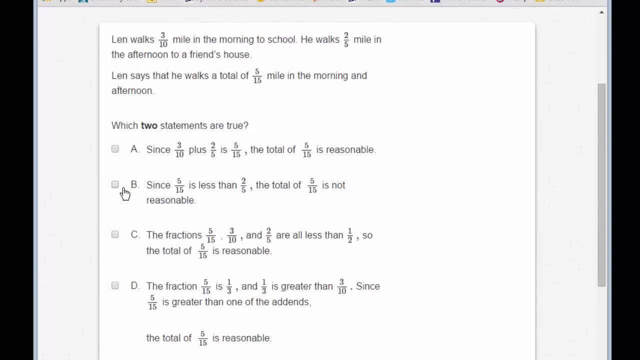 Be sure, before you move on, to select at least two. Don't select three, don't select four and don't only select one. Answer the entire question and be careful about reading the instructions, As I said. that should be familiar to you from the ELA. 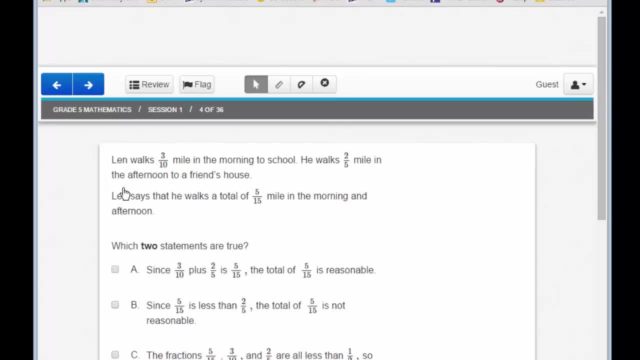 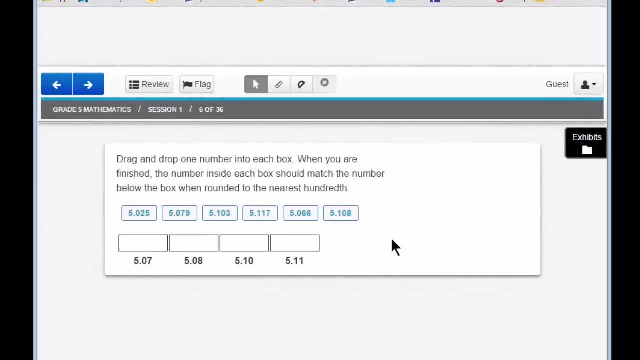 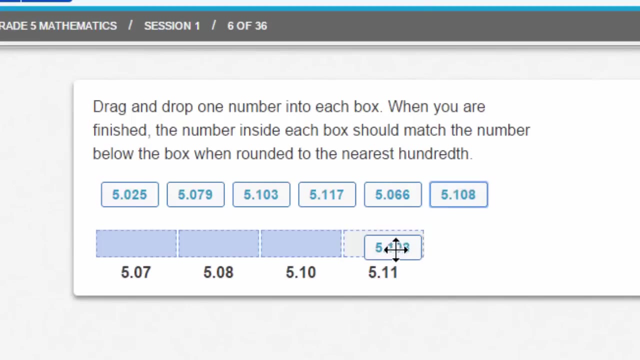 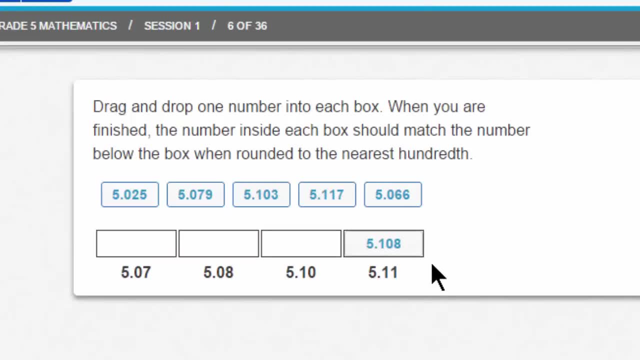 appropriate blanks. If you decide that that is not correct, you can move it back out. Let's look at this question. Drag and drop one number into each box. When you are finished, the number inside each box should match the number below the box. 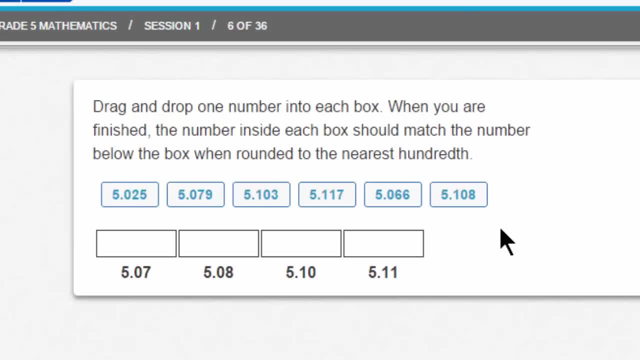 when rounded to the nearest hundredth. So 5.108 rounded to the nearest hundredth is 5.11.. That's my answer. 5.066 rounded to the nearest hundredth is 5.07.. 5.079 rounded to the nearest hundredth is 5.107.. 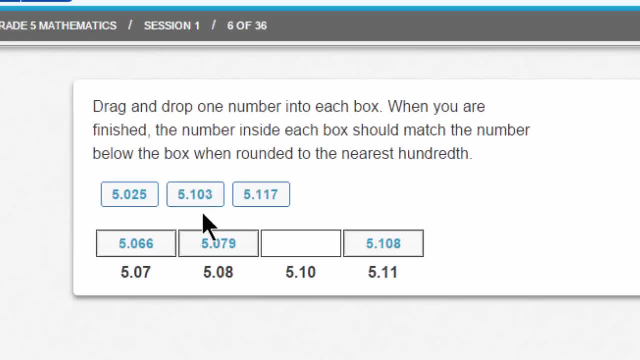 5.108 and 5.103 rounded to the nearest hundredth is 5.10.. You can see that I have two answers left over, but I have completed this question. Dragging and dropping works in much the same way. it works on the ELA test and, as you've. 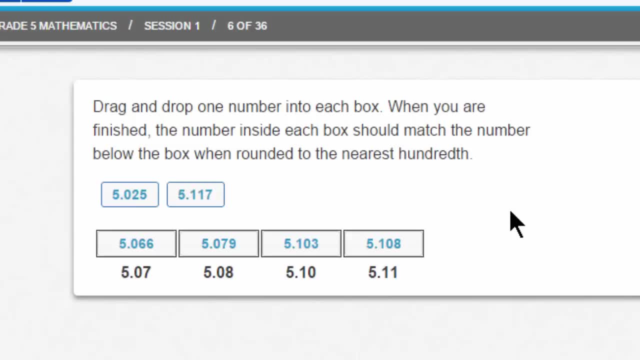 probably mastered it there. you'll master it here easily. Let's move on to a math test. Let's move on to a math test. Let's move on to a math test. Let's move on to a specific tool. Move to question 9.. 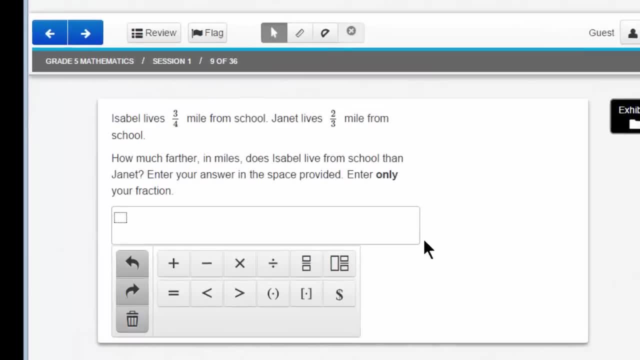 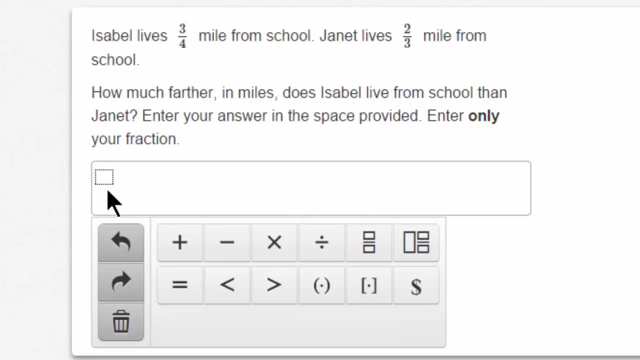 Question 9 looks quite a bit different. It has this text field, this box that you must enter your answer into. but you'll also see this little dotted line box here. This shows that you're working with a powerful math tool called the Equation Editor. 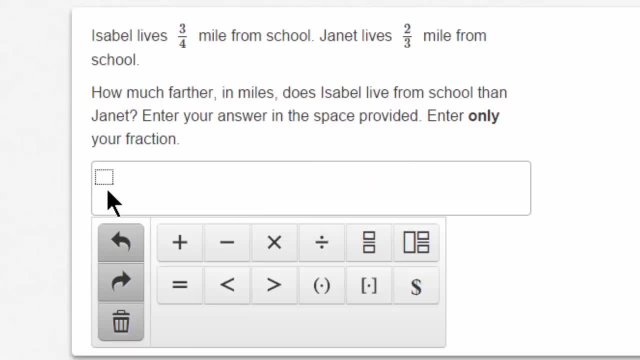 Let's read the question to find out what we're doing doing. Isabel lives 3 quarters of a mile from school. Janet lives 2 thirds of a mile from school. How much farther in miles does Isabel live from school than Janet? 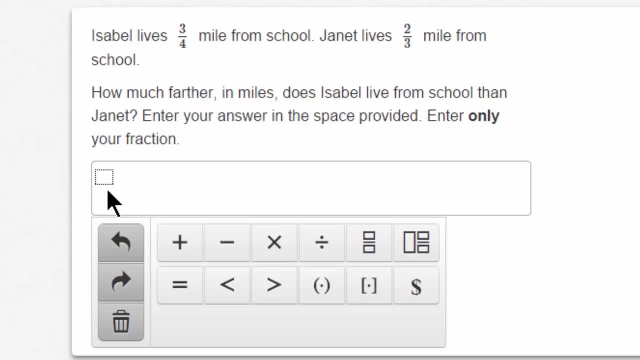 Enter your answer in the space provided. Enter only your fraction. In a simple text field, entering a fraction could be difficult. The equation editor will help you enter an equation or a special character or number, like a fraction or a mixed number. 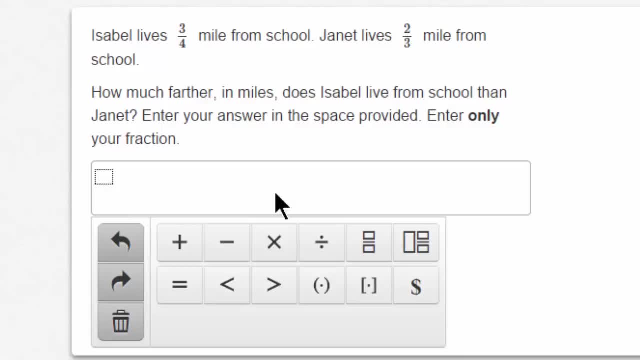 or a greater than or less than equation. These buttons here will tell you what you are using. This is the fraction button And as you hover over it you can see fraction different from the one to the right, which is a mixed number. 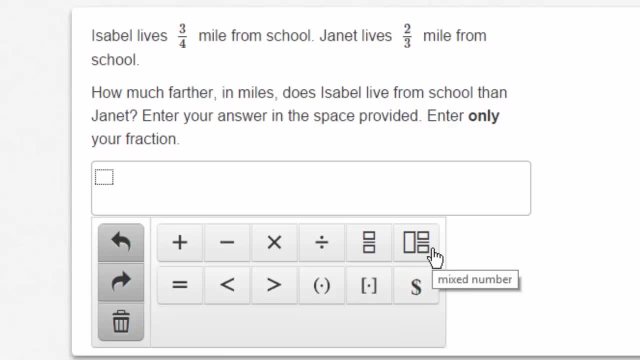 Let's see what our answer might be. You might be a little bit confused as to how to work this question, But you will have access to blank paper on the test, So if you have blank paper next to you, you can work out the problem. 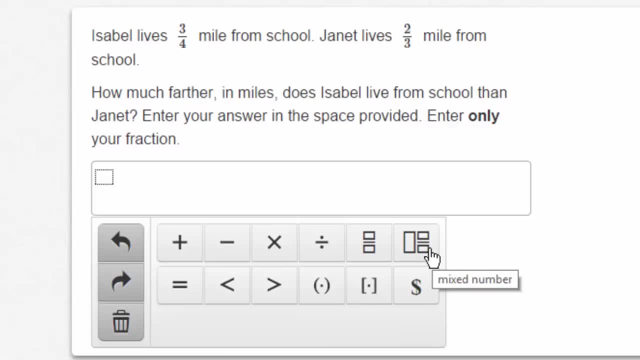 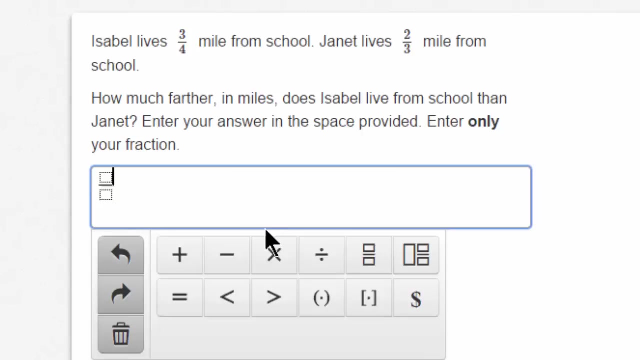 Take a moment and see if you can find the answer. Did you come up with the answer 1, twelfth, Excellent, Let's try entering that. Click on the fraction button. You'll see that my one dotted line square turns into two. 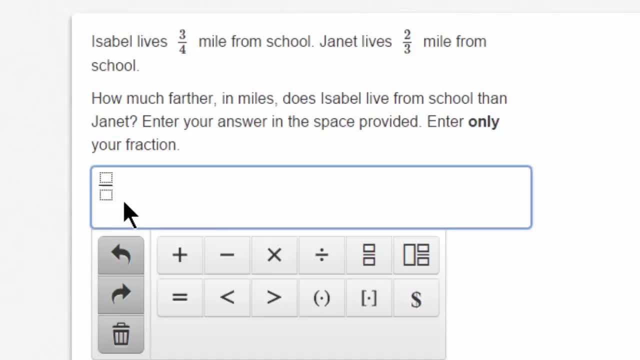 The dotted line square shows where your number will appear. I'll type the one And that appears in the top. Now if I type twelve, oh, it still appears in the top. Let's use the backspace button. So how do I enter the twelve? 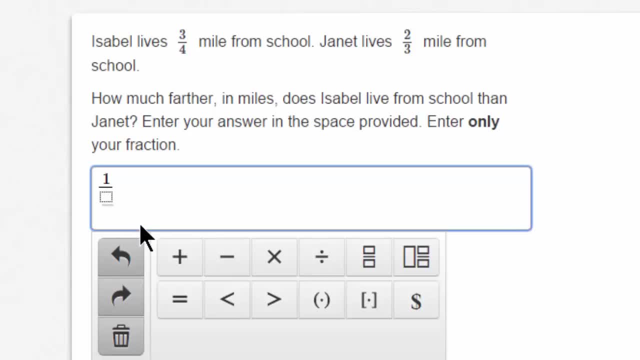 I can do this in two ways. I can click down here, and that's the twelve, Or I could, if I'm up here in the top, tap the tab key And that will move me down to the bottom. Clicking or using the tab key will help you move through easily. 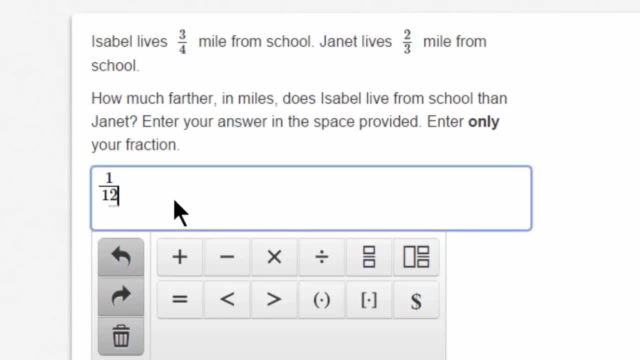 This question, once again, is now answered without any submit or save. The equation editor will give you powerful access to special math characters. Use those math characters to enter the answer, as you've been taught by your math teacher. Practice with this for a moment. 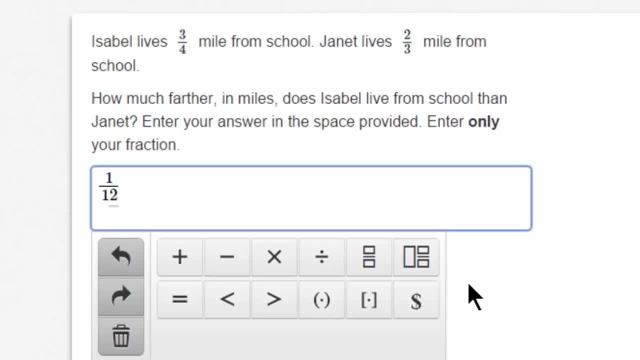 Perhaps practice with mixed numbers, absolute values or parentheses. Become comfortable with the equation editor. And now let's move on to the next question. Let's move to item ten. Are you ready to move on? Then let's move to item ten. 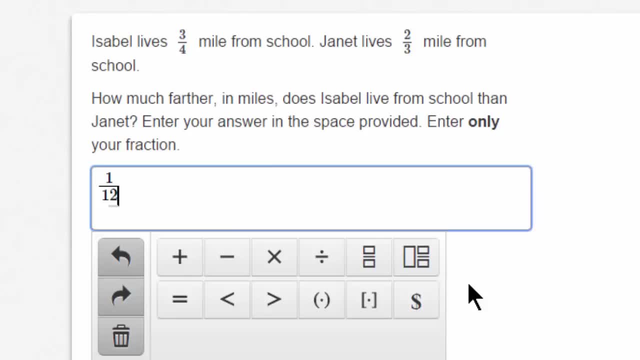 Item ten asks a question that you should answer in the box, as we've seen before. But let's try something a little bit different. We won't answer this question right now. Instead, I'd like to use it to practice with you. 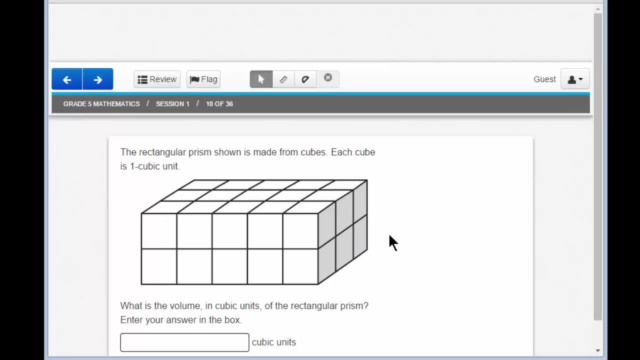 and to help you learn how to use the equation editor. So let's start with the question. Let's try something a little different. We won't answer this question right now. Instead, I'd like to use it to practice with you. 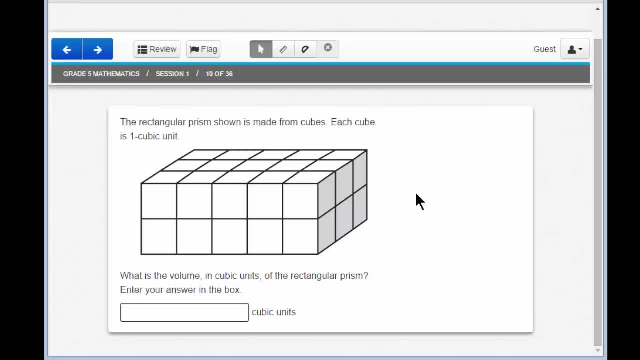 and to help you learn how to use the equation editor. Instead, I'd like to use it to practice with you and to help you learn how to use the equation editor. Instead, I'd like to use it to practice with you, to practice a couple of tools that you've seen in the toolbar. 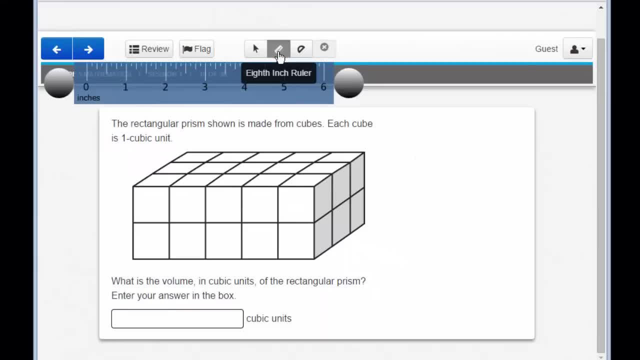 Look up here. You can see a ruler and a protractor. You can see a ruler and a protractor. Let's try the ruler. When we click on the ruler, a ruler appears that we can click and drag around the screen. You'll see that it's slightly transparent. 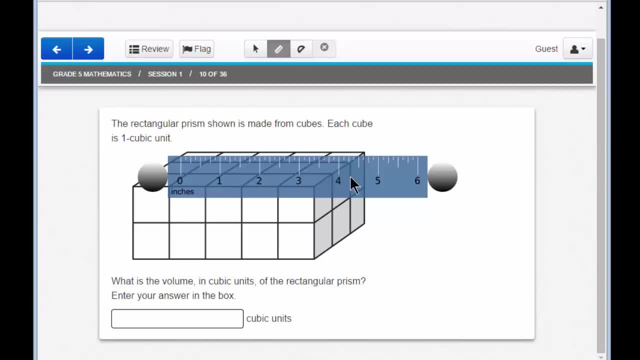 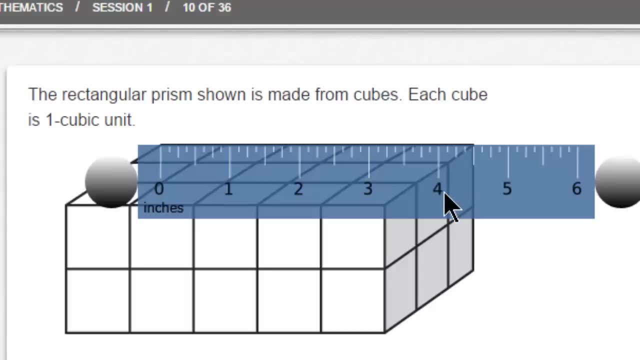 and that will make it easier for you to measure lines. and that will make it easier for you to measure lines. Let's try measuring the back line. I can line this up and see that this back line measures about 4 1⁄2 inches. 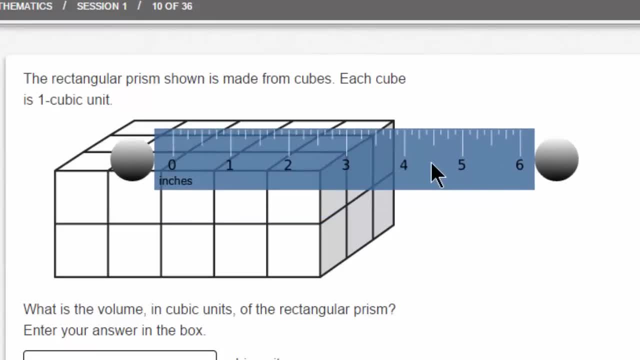 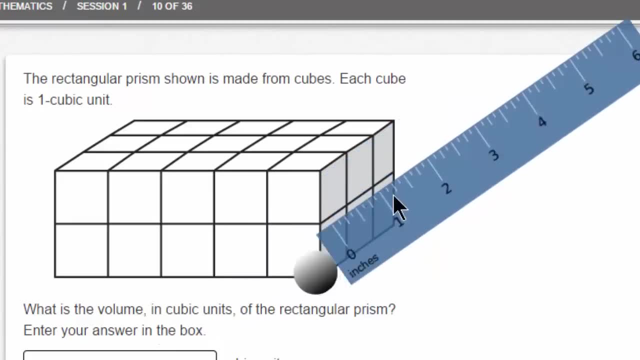 What if I wanted to measure an angled line? That's pretty difficult unless I grab a circle and angle my ruler. Then I can move the ruler to where I need in order to measure, and I can see that this is approximately 1 1⁄2 inches. 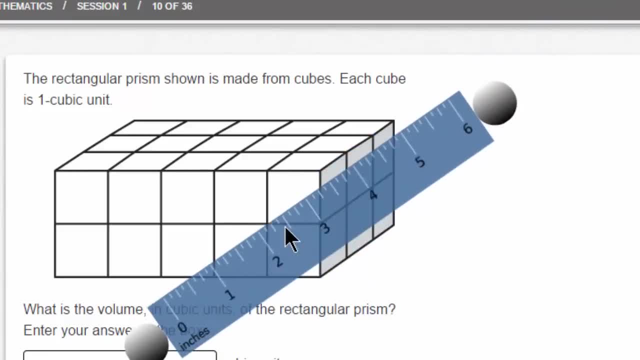 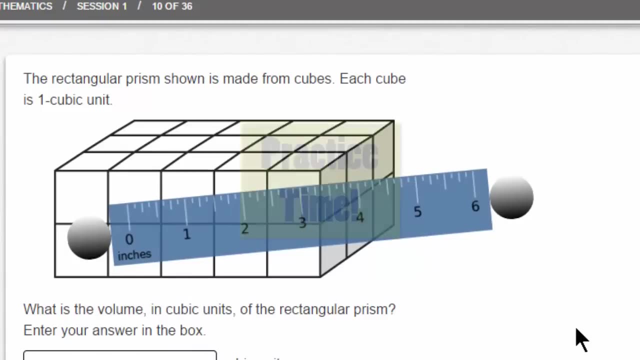 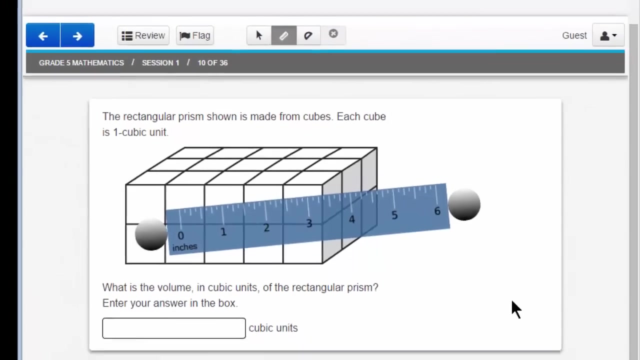 Easy enough right. Move the ruler around and practice with it for a moment. Try to measure different lines, see how long they are and see if you can master using the ruler's angling function. When you're finished, turn the ruler off by clicking on the Ruler button. 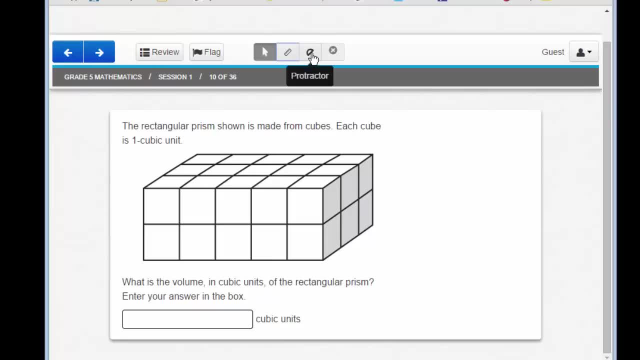 Now let's try. the next tool. Right next to the ruler is the protractor. Click on the protractor and move it around the space, just as you would the ruler. You can use a protractor to measure the length of the ruler. 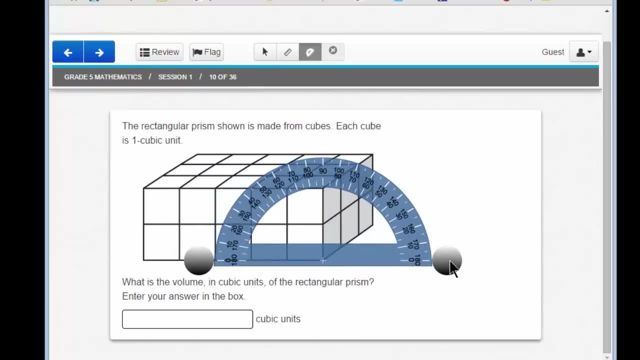 You can also use a protractor to measure angles when the question requires you to, And, just like the ruler, you can angle the protractor if you wish. Try moving the protractor around as well. See how well you might be able to measure angles in this image.